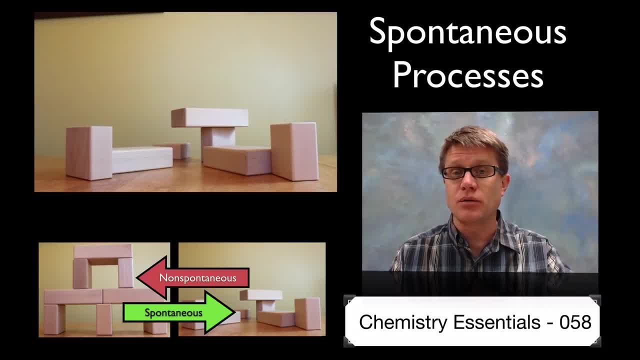 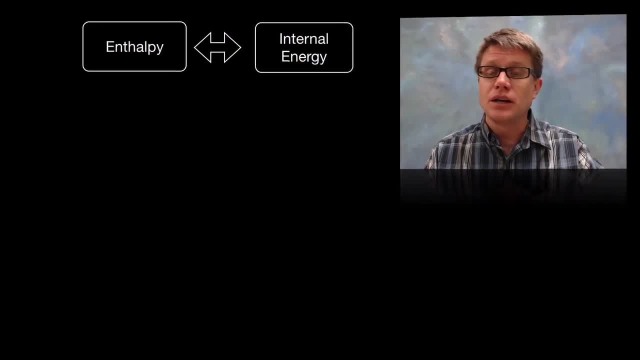 It's not magically going to move in the other direction And so in the other direction, that would be a non-spontaneous reaction. It's not going to occur. It's statistically impossible for that to occur, And so, as I talk about spontaneous reactions, I'm going to treat 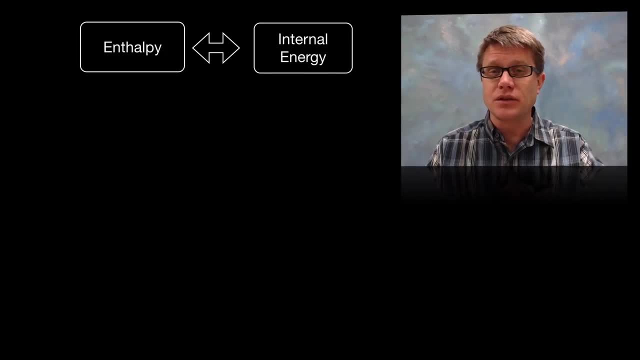 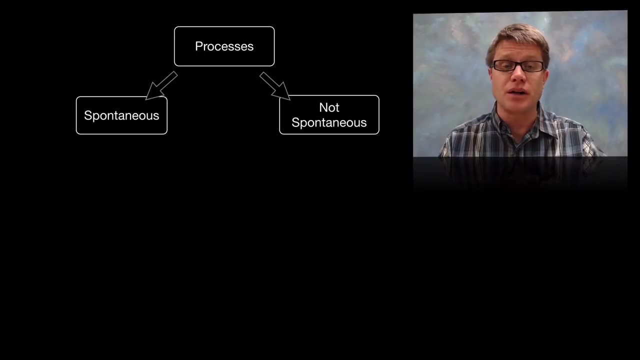 the words enthalpy and internal energy the same. There are slight differences, But we're just going to treat them as synonyms. And so in processes we're going to talk about reactions. We're going to talk about reactions In processes. we can either have spontaneous or non-spontaneous processes. We can know that. 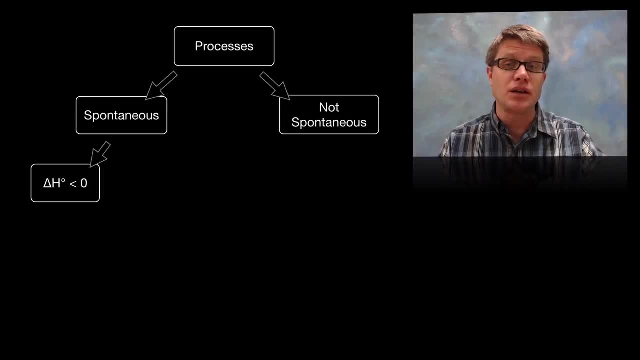 it's a spontaneous process right away if we ever see a decrease in enthalpy and an increase in entropy. Now, if you don't know what these two things are, I'll put links to videos about both enthalpy and entropy. But if we ever see a decrease in that amount of internal 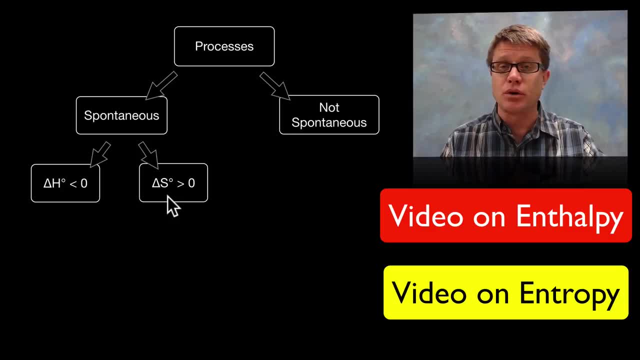 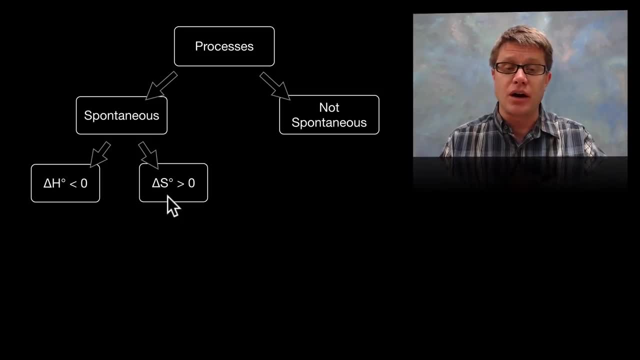 energy and an increase in that randomness or that dispersal, of that matter. we know that it's a spontaneous reaction In any spontaneous process. we can either have spontaneous or non-spontaneous reactions. In any spontaneous process it's going to favor the products or the things that are. 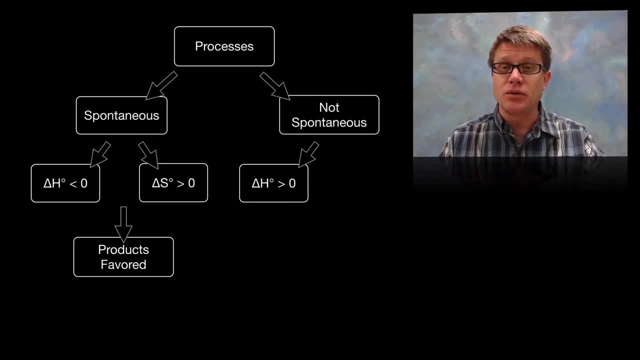 created in that process. If it's non-spontaneous, we can know right away. if we see an increase in enthalpy and a decrease in entropy, We know that that's going to favor the reactants and it's going to be non-spontaneous. And so how do you know if we're favoring the products? 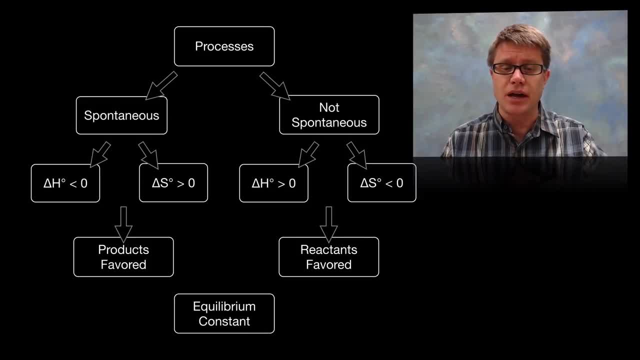 or the reactants. We can use something called the equilibrium constant to figure that out, And I've got a little model that shows you that If we ever see an equilibrium constant greater than 1, we know that that's going to be non-spontaneous, We know that it's going. 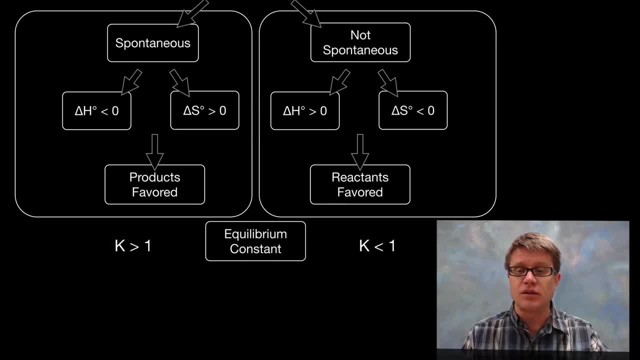 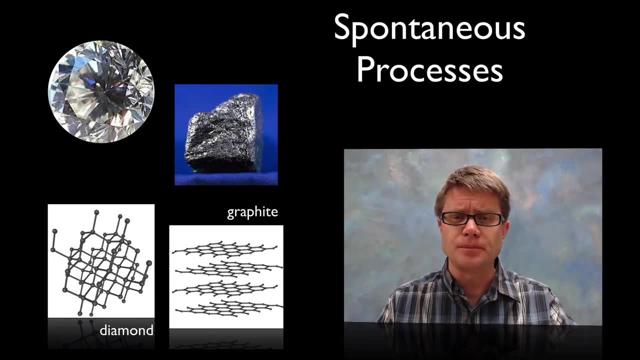 to favor the products and it's going to be spontaneous. If it's ever less than that- less than 1,, we're going to see a non-spontaneous reaction. Now the thing that's tricky about a spontaneous reaction is that it just doesn't occur magically. Sometimes it can occur over. 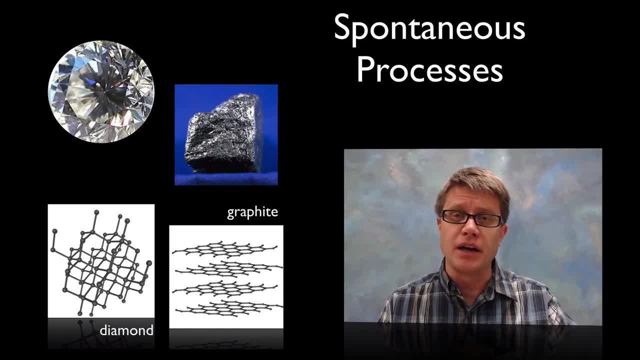 millions of years, And so you probably know that graphite can be turned into a diamond, but it takes a huge amount of energy and it takes a huge amount of pressure, And so that's going to be a non-spontaneous process. It just doesn't occur on its own without external 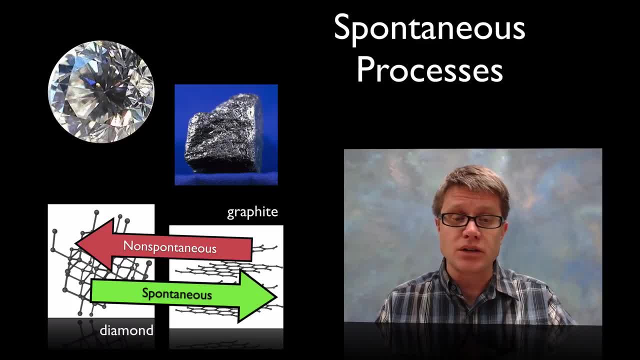 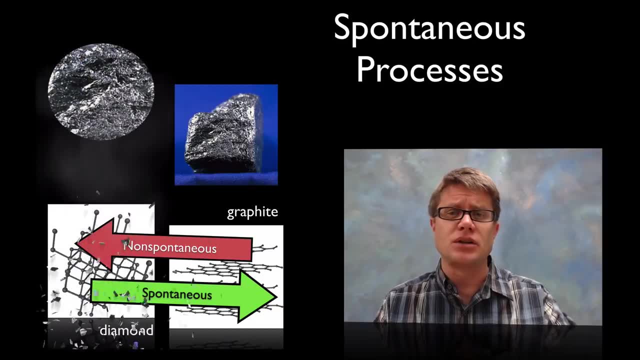 energy. It takes a huge amount of energy. But if that's in one direction, in the opposite direction we're going to have a spontaneous reaction. But you know that a diamond just doesn't break down into graphite. It takes millions of years for that to occur, And so spontaneous process is probably a bad term. 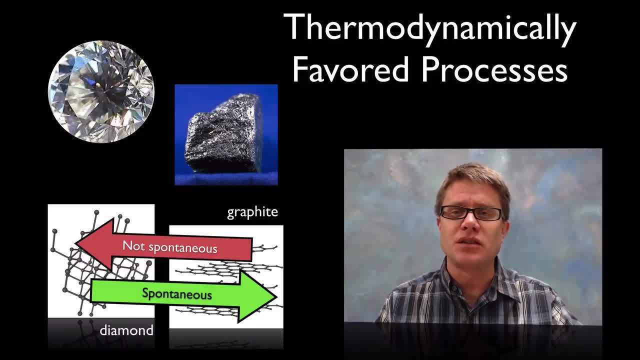 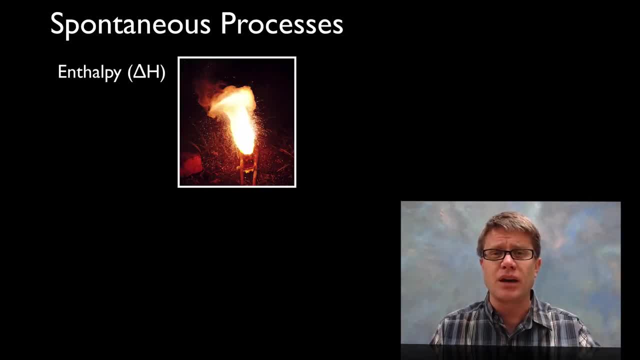 It's better to use a thermodynamically favored process. That just is too much of a mouthful. And so if we're looking at a spontaneous process, one of the first clues is to look at the enthalpy, which is the amount of internal energy, And if we ever have a change in enthalpy, that 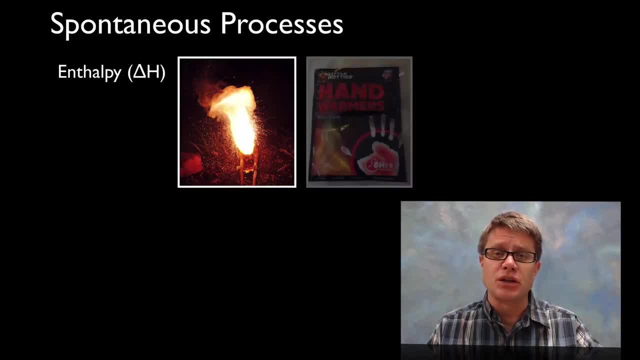 is negative, we know that that is probably going to be spontaneous reaction. So if we were to look at a thermite reaction, it's exothermic, It's giving off that energy. That means our reactants have more energy than our products. If we were to look at the rusting of iron, like you, 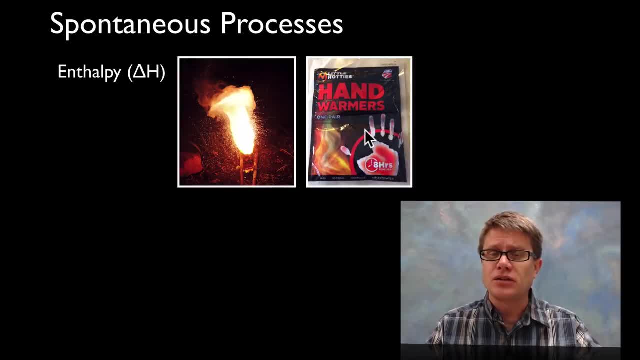 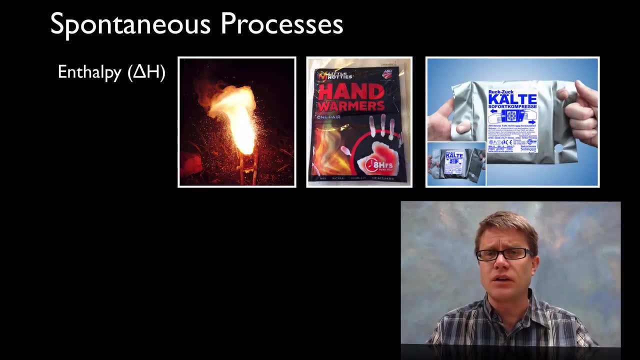 do in the hand warmers, we have a negative enthalpy change, And so that's a clue that this is going to be a spontaneous reaction, But sometimes we'll have reactions that occur on their own, but they, instead of giving off energy, are actually consuming that, And 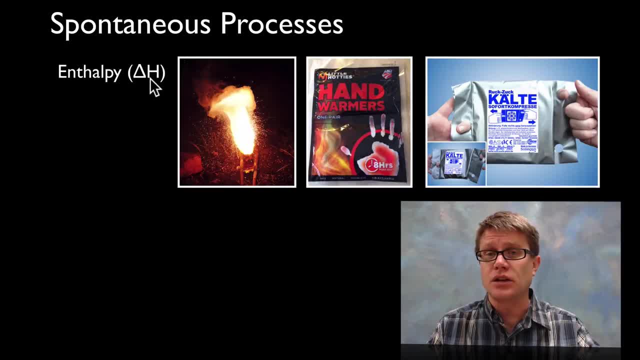 so if we were to look at this cold pack right here, that means that our delta H is going to be a positive value, So it's going to be an increase, And so we can't just look at enthalpy itself. We have to add entropy to the equation. So imagine if I had these two. 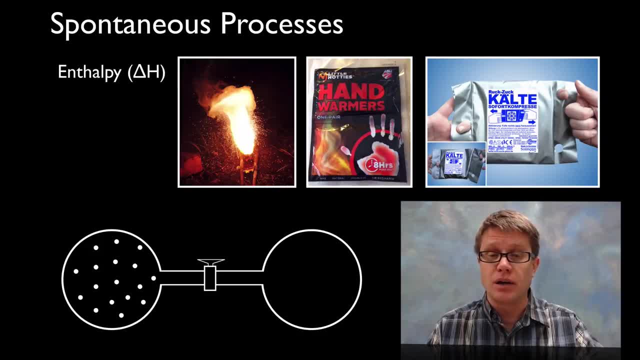 spheres. On the left side, we've got gas. On the right side, we have a vacuum, And now we're just to open it up. what's going to happen to those molecules? Well, they're going to move from the left to the right side. Is there any change in temperature? No, And so what? 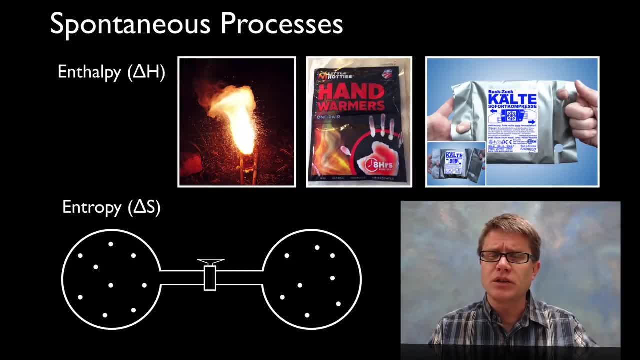 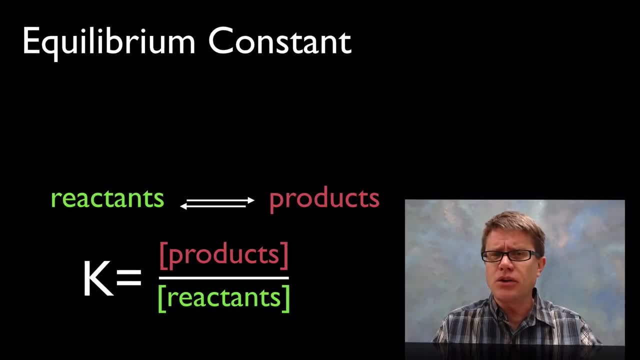 we're seeing there is a change in entropy, And so if you're looking at a spontaneous process, you don't want to only look at the change in enthalpy, You want to look at the change in enthalpy, You want to change in that entropy as well, And so to figure out, 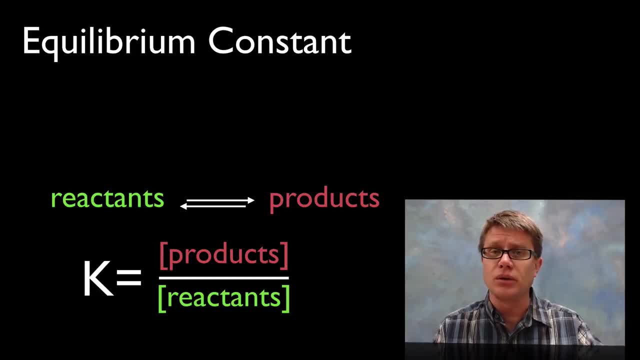 if we're favoring products or reactants, we can use a term called the equilibrium constant, Which really works with reversible equations, But this will work right here. So if we imagine we have reactants and products, the equilibrium constant is simply the concentration of products. 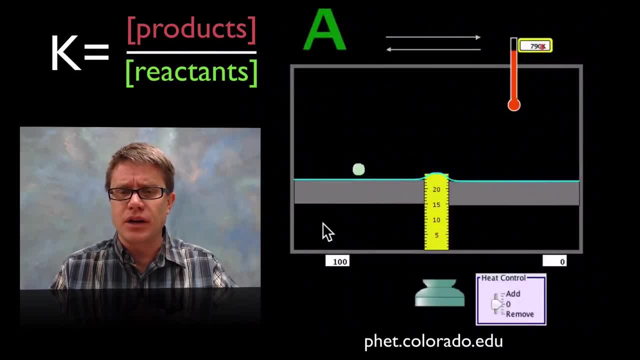 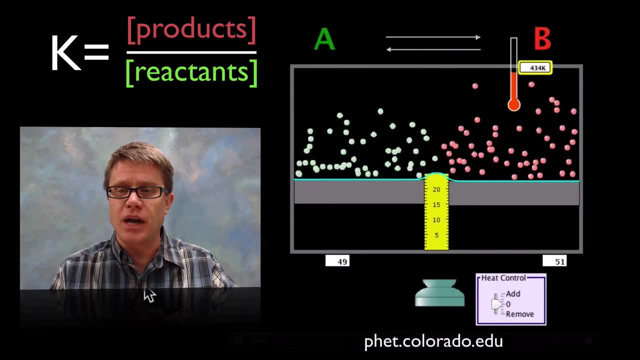 divided by the concentration of reactants. And so let's look at this first scenario, And this is a PHET simulation. I'm going to put some molecules over here on the left side, And so they're going to spread out, And then they're going to be acted on by gravity. They're 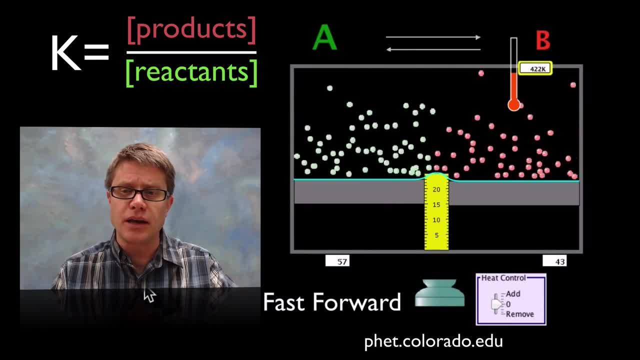 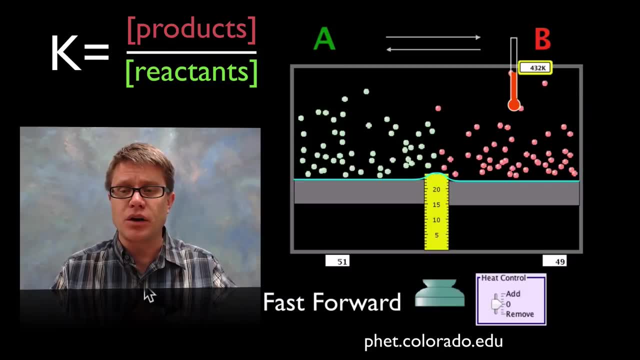 going to bounce back and forth. I started with 100 of those molecules on the left side. They're randomly dancing back and forth And so as they move to the right side we're changing color, And so we can represent those as products. So if we look at how many I have on the left, 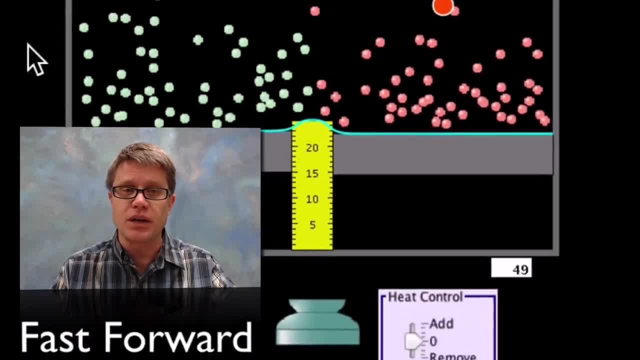 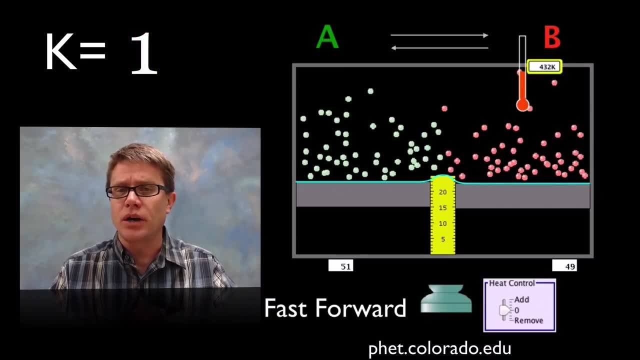 side and the right side. On the left side, I have 51.. On the right side, I have 49.. If I were to divide my products by my reactants, 50 over 50, we would say that my k value is right around 1.. And so we're going to be at equilibrium. In other words, we're going to 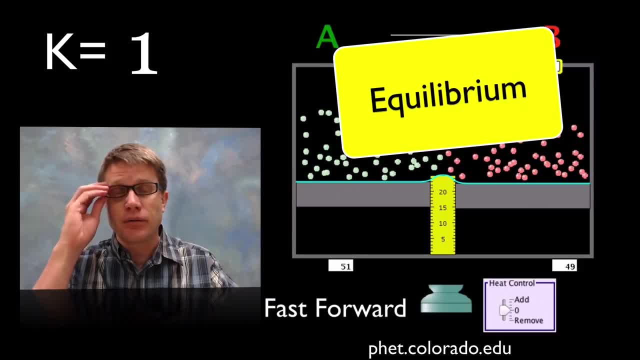 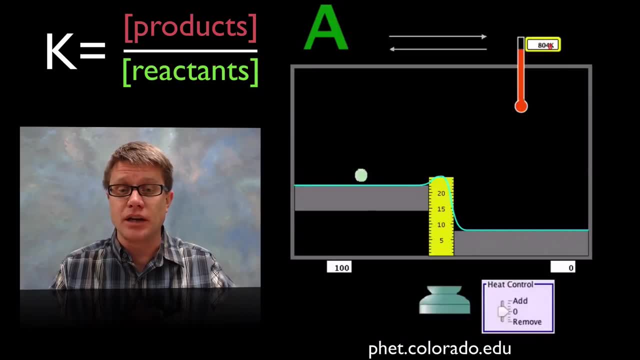 we're not favoring either reactants or the products. Now, if we look at this next simulation right here, I'm going to change it a little bit. I'm going to put the ones on the left side and give them a little bit more gravitational potential energy, And let's start that going. 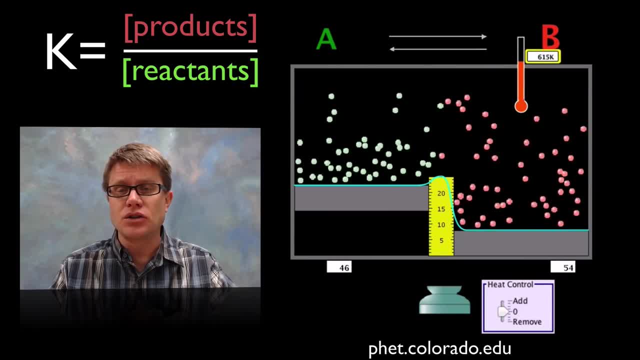 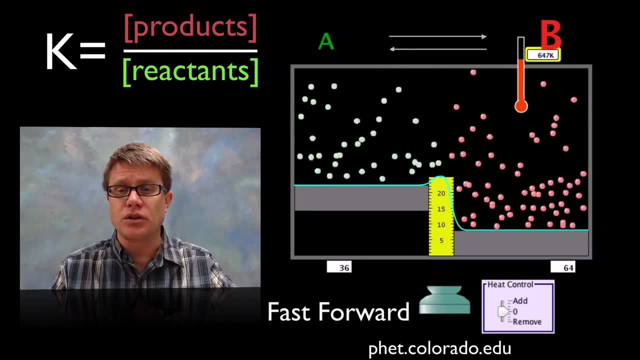 And so, again, those molecules are bouncing around. You can see that the energy on the reactant side is actually higher than the energy on the product side, And so that's pushing those molecules over to the right side, Or it's favoring those products If 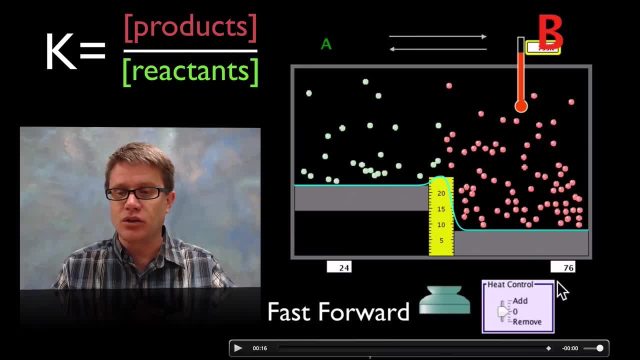 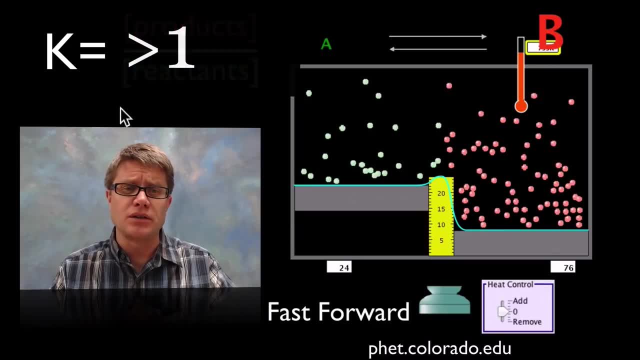 we speed it up and let it run for a while. you can see now that I have 76 molecules: 26 molecules on the right, 24 on the left. So if I were to put 75 over about 25, my k value is going to be around 3.. And so that means it's going to be greater than 1.. So we're 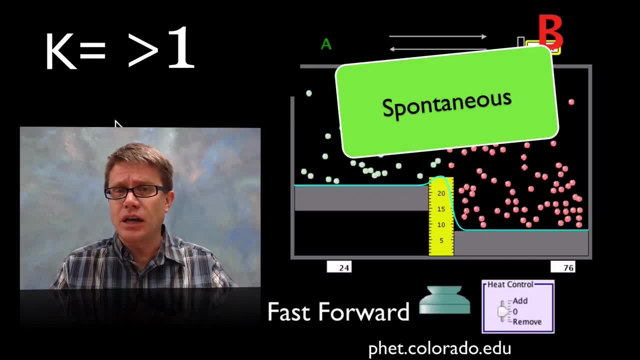 favoring products in this case, And so that's going to be a spontaneous reaction in this case Or a spontaneous process pushing it to the right. What have we done? We've seen a decrease in the enthalpy or decrease in the energy, And if you look at it carefully, 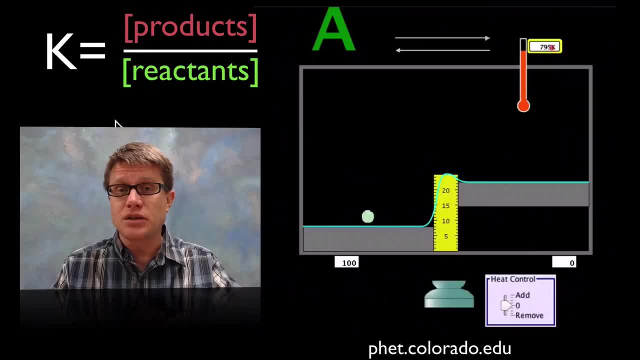 you can actually see an increase in entropy as well. Let's go in the opposite direction. Now I've given less energy on the left side. If we let this run for a little bit, It's hard for them to get up to the right side. 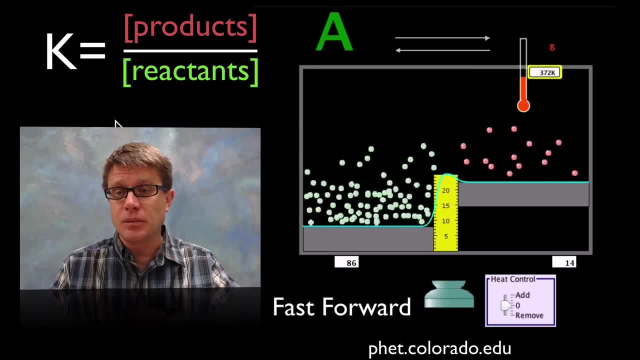 It's hard for them to become products, And so let me speed this up a little bit and we'll watch it change over time. You actually see less entropy in this model right here. Less change because it takes more energy to move to the right side. If we were to figure out. 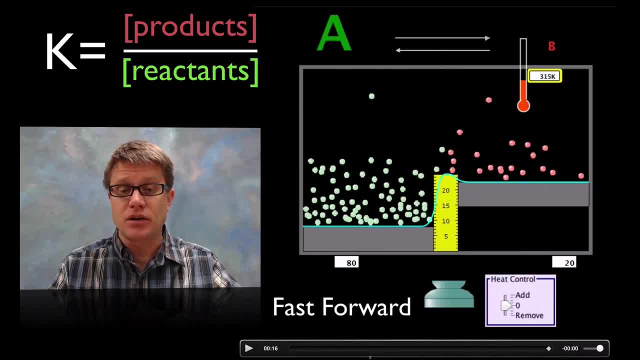 the k value. now our products are at 20.. Our reactants are going to be at 80. So if I were to figure out my k value, it's around 0.25.. And so it's going to be less than 1.. So if 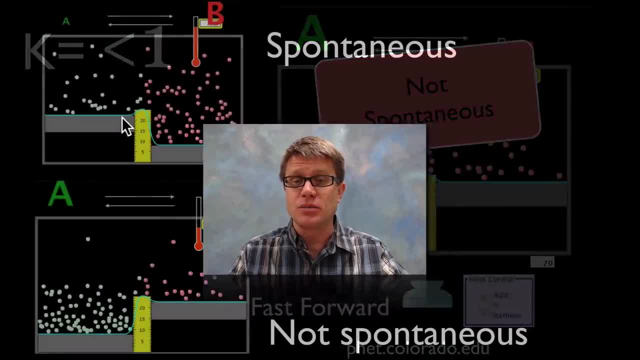 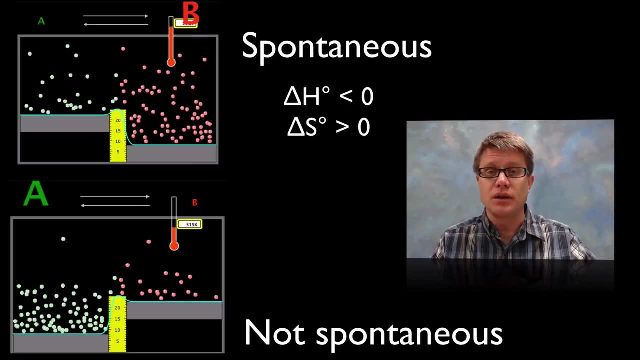 my k value is less than 1, that tells me that this is going to be less than 1.. And so I'm going to find this is probably a non spontaneous reaction. So in a spontaneous reaction, you know it's spontaneous right away. if you see these two things, If you see a decrease in 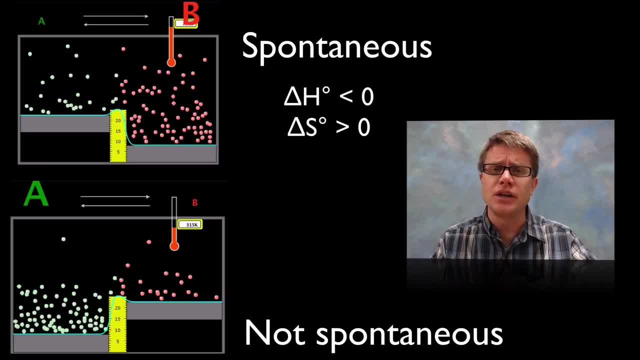 enthalpy or decrease in that internal energy, And you see an increase in entropy. it's non spontaneous if we see the opposite of that, In other words, if we see an increase in enthalpy. In other words, if we're looking at an endothermic reaction And we see a decrease in entropy.